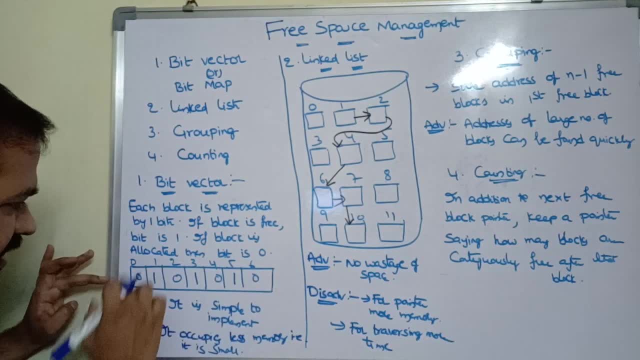 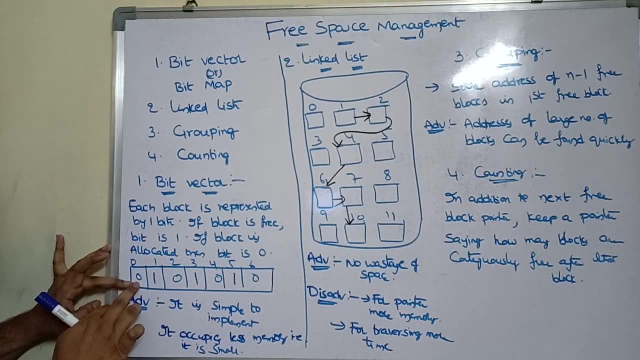 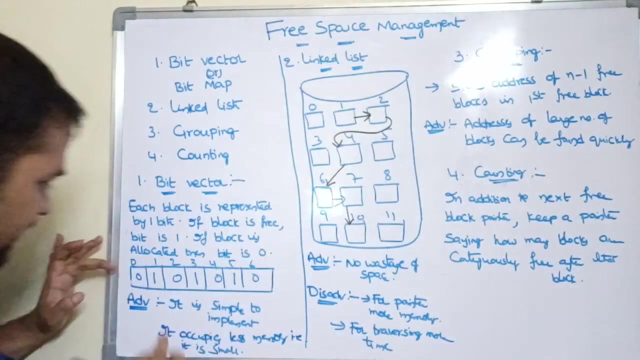 If the bit is 1, then it specifies that the block is occupied. So let us assume that we have seven blocks, from 0 to 6. Here, 0th block bit is 0. So it specifies that this block is allocated. So likewise, second block is allocated. Fourth block is allocated. Sixth block is allocated. 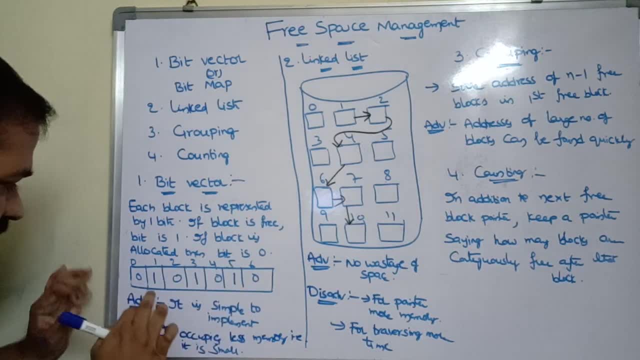 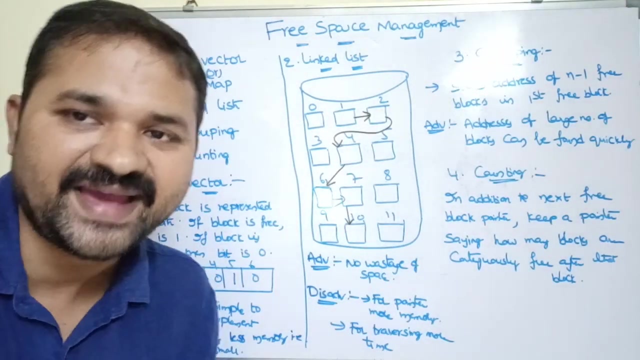 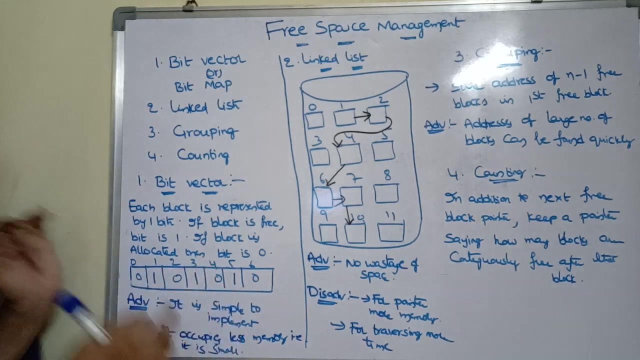 Various first block, third block and fifth block are set to 1.. So this one specifies that first block, third block as well as fifth blocks are allocated. So operating system can use these blocks for allocating memory to the files. So 1 specifies that the corresponding block is free. 0 specifies that the corresponding block is already occupied. 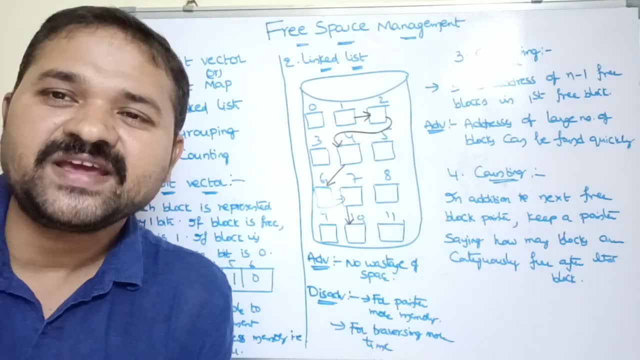 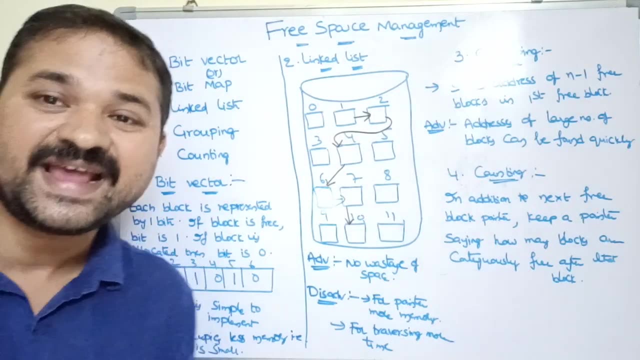 So the advantage of this approach is that it is very, very easy to implement this approach. So it is very, very simple to implement this approach and it occupies very, very less memory. That is, it is very, very small. Why? Because in each block, equal memory. 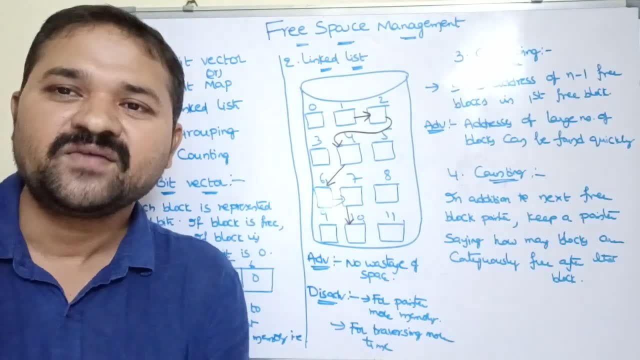 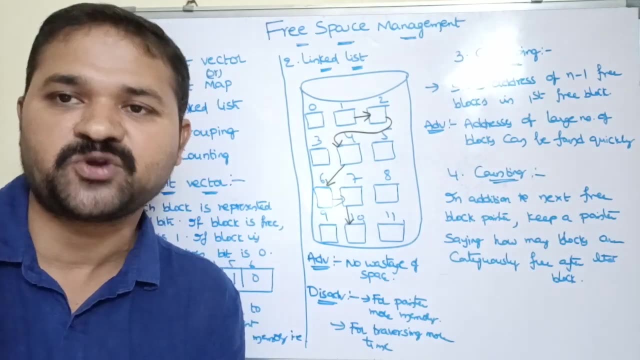 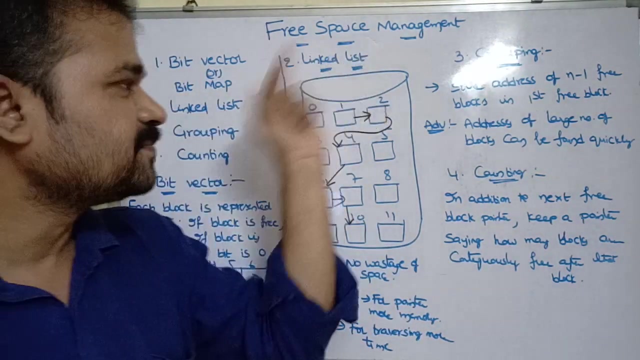 have to maintain whether it is occupied or empty with the help of a single bit, one or zero. so one specifies that block is free, whereas zero specifies that block is occupied. so it is very, very small. it occupies less amount of memory. let's see the second approach, that is nothing but link list. 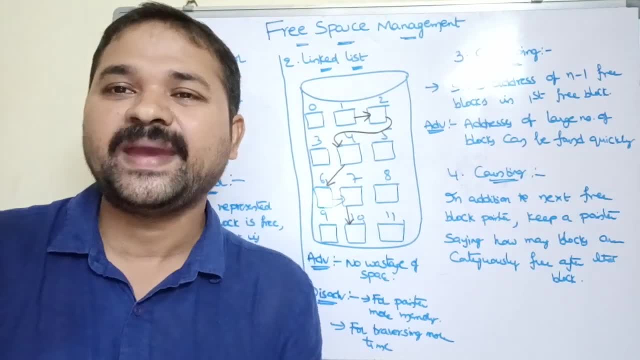 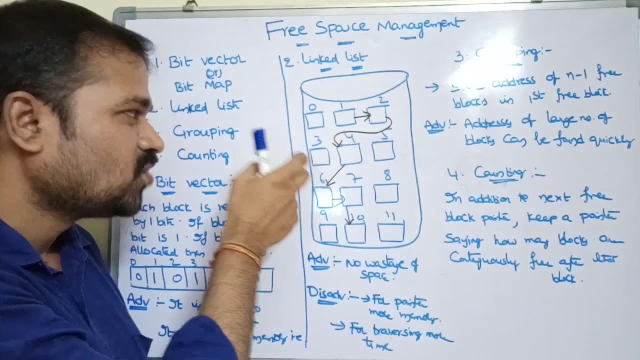 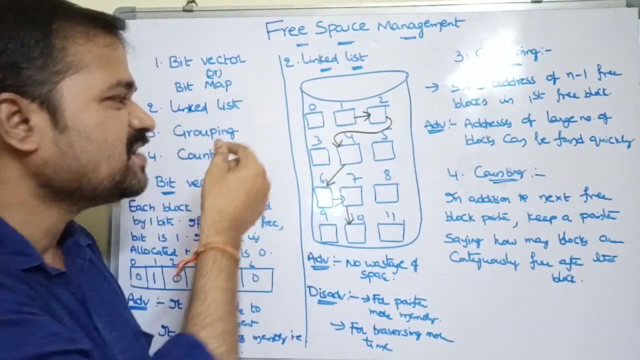 here we maintain a link list in order to maintain the free blocks. so here the first block is one. so this one is nothing but header block. why? because we know that in a linked list the first node is known as header node. so we have to store address of the first node in a variable. 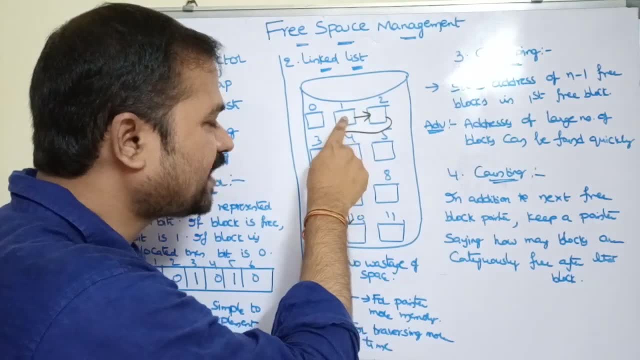 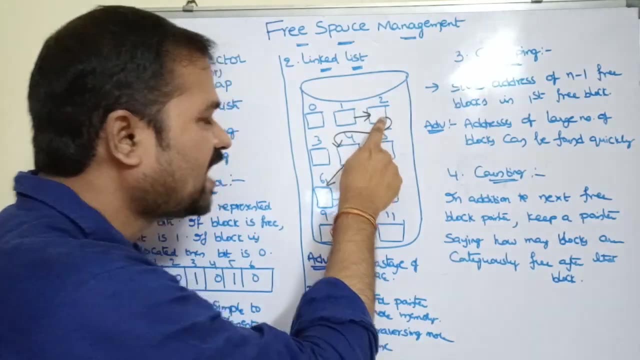 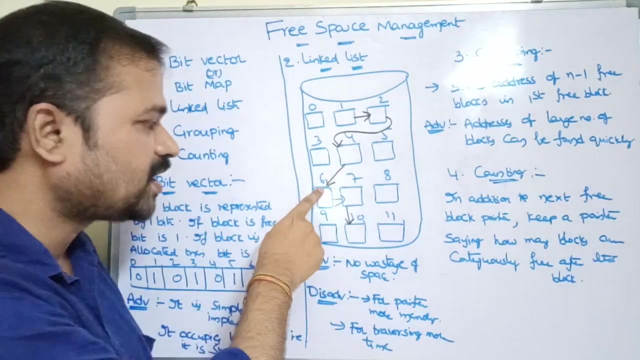 called head, and the second and the first block contains the first block. pointer field contains address of the second block. next to second block pointer field contains address of its next block. that is nothing but fourth block. fourth block pointer field contains address of its next free block, that is sixth block. sixth block pointer. 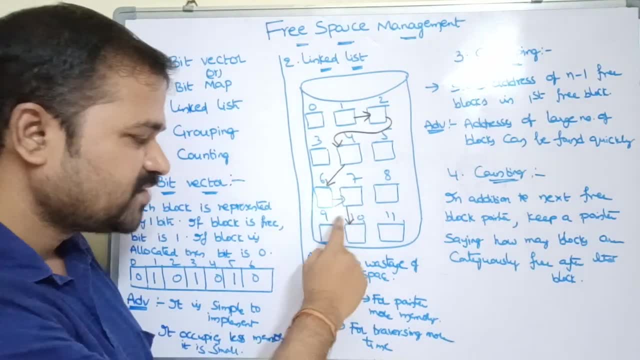 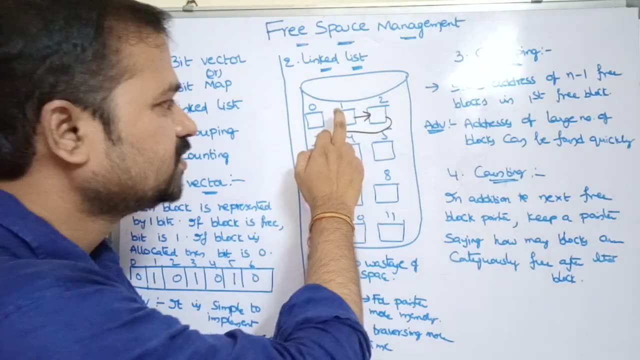 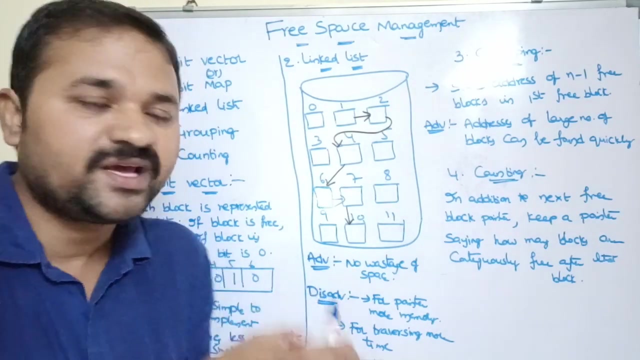 field contains address of its next free block. seventh, various. what is the last block? tenth block. so tenth block. next field is none. so here we have a linked list of so one, two, three, four, five, six, six free blocks. so totally we have six free blocks, so here we are maintaining those six. 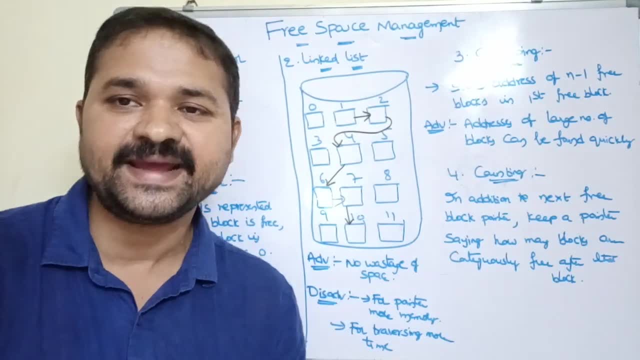 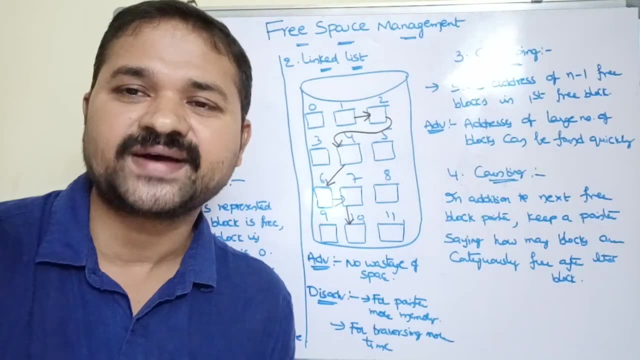 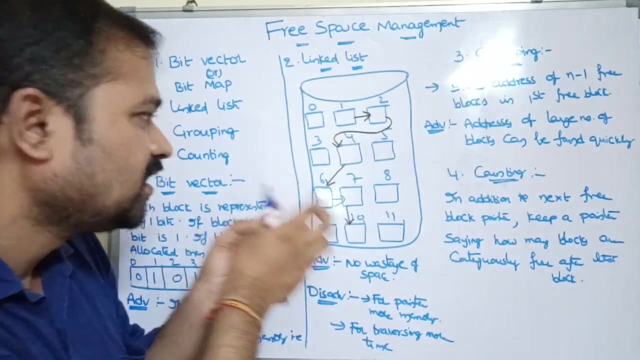 free blocks with the help of a linked list. okay, so this is the second approach. let us analyze the advantages and disadvantages. the first advantage is: here: there is no wastage of space here. there is no need to have extra space here. why? because already we have some blocks in those. 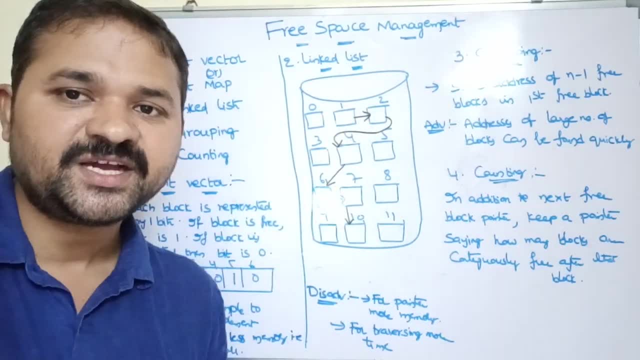 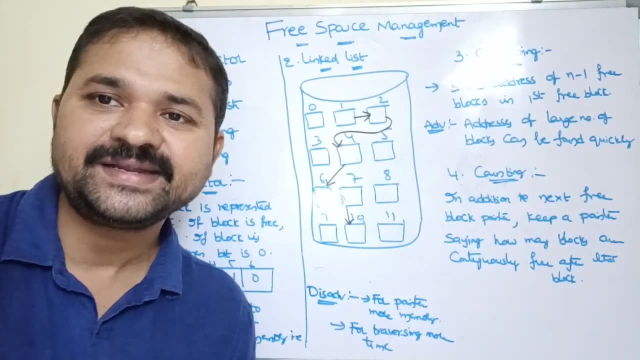 blocks only. we are maintaining the links. now let's see the drawbacks of this approach. the first drawback is here: in each block we have to maintain a pointer. that pointer contains address: all pizza next to free block. so in order to store the pointer, we require much amount of memory. 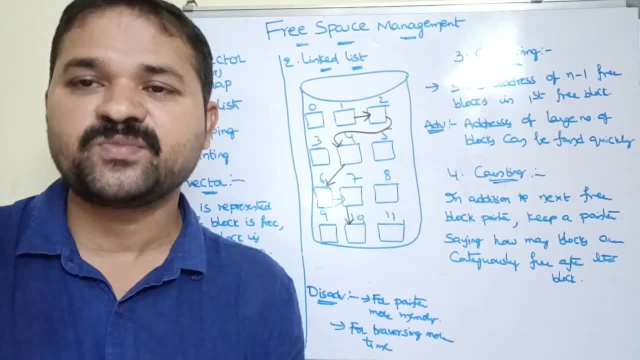 and the second potential advantage: if we want to store the entire row of the in box of each block- and the first drawback is here- in each block we have to maintain a pointer. that pointer contains it. second problem is for traversing. it will takes large amount of time. let us assume that here we. 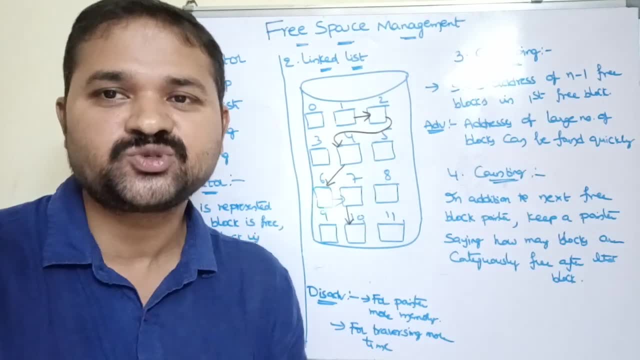 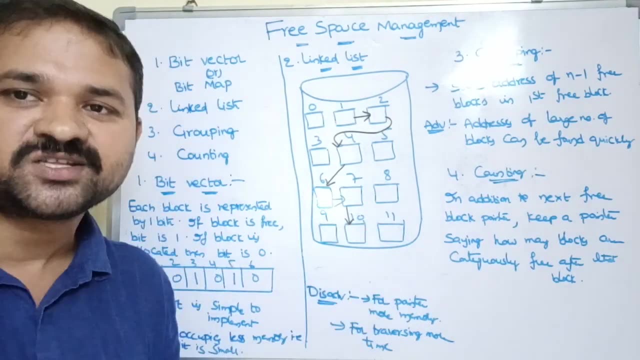 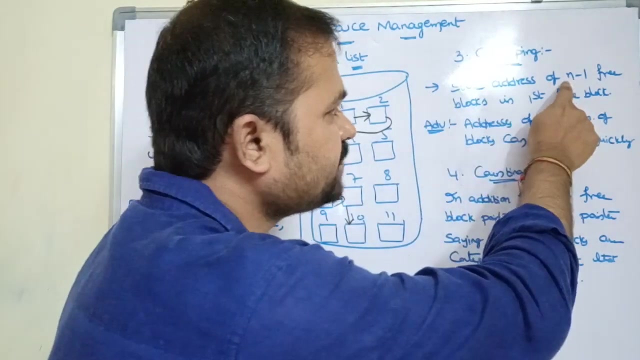 have 100 free blocks. so if you want to traverse to the last block, then we have to traverse all the 99 blocks before 100 block. okay, so these are the problems here, and the third approach is grouping. so let's see what is a grouping here. store address of n minus 1 free blocks in the first free block. 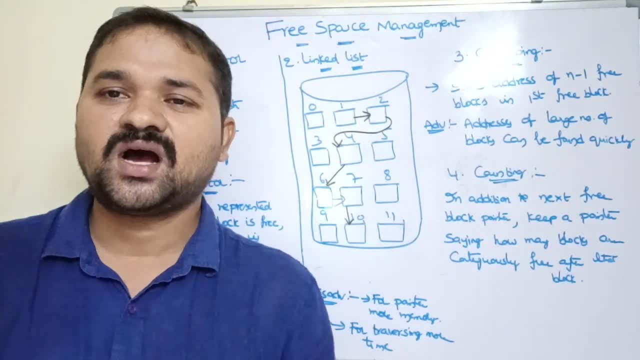 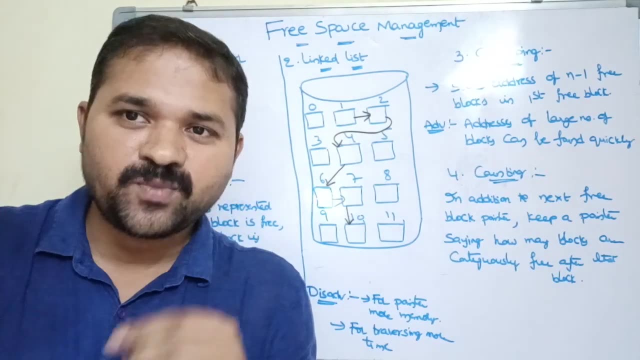 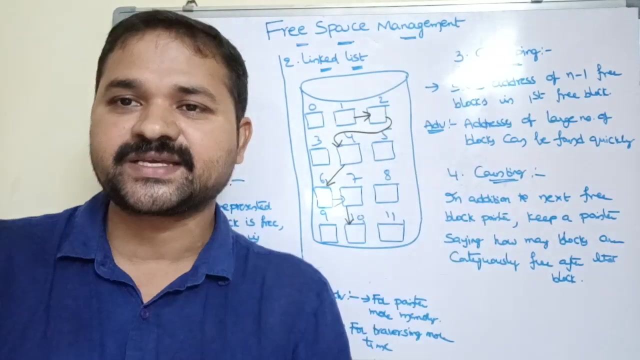 so in link-list, what we are doing is, in each block we are maintaining a pointer. that pointer contains the address of its next free block. next free block contains a pointer that contains address of the third block, like that, whereas in this approach, what we are doing is we have to. 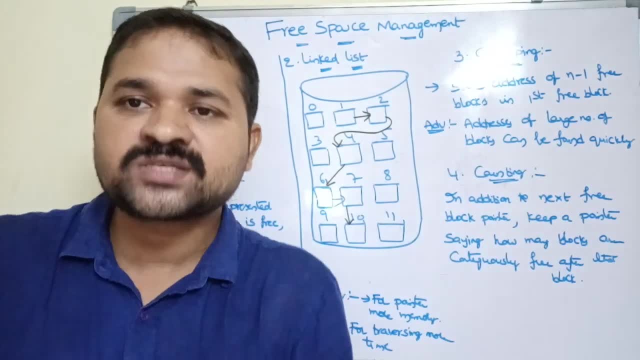 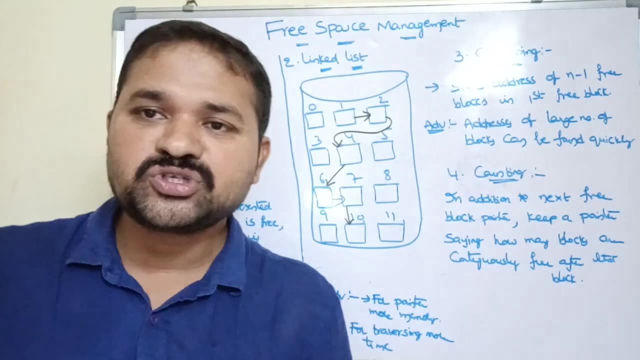 address of n minus 1 free blocks in the first block. okay, so let us assume that we have 10 free blocks, so in the first block only we have to store the relatedgood points in the next three blocks only. so we are maintaining a pointer in the 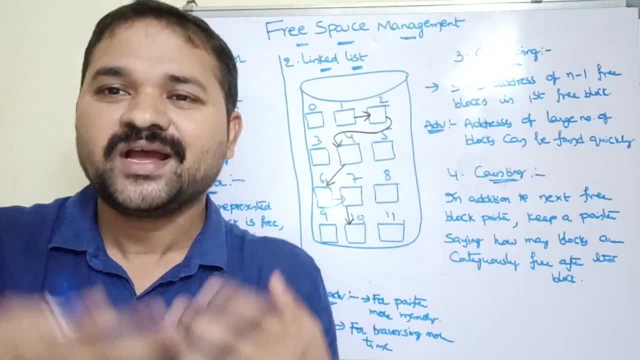 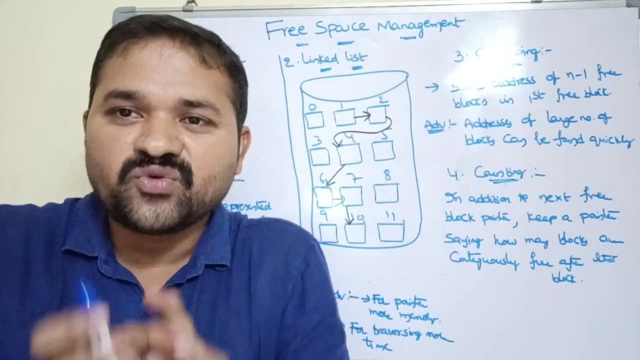 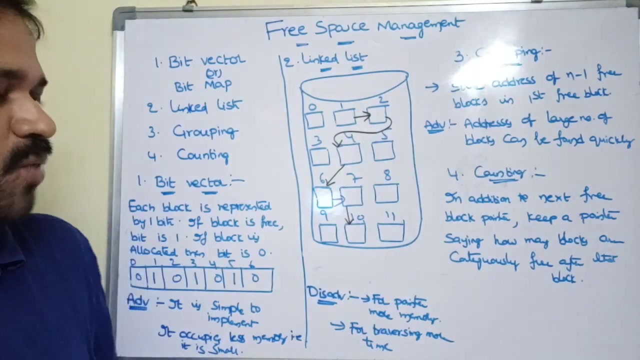 nine blocks addresses, so that we can get large number of blocks very, very easily. so that is the advantage of this approach. so that is nothing but grouping. so we are grouping several blocks into one block. okay, now let's see the last approach. that is nothing but counting in addition to the next free block, pointer. 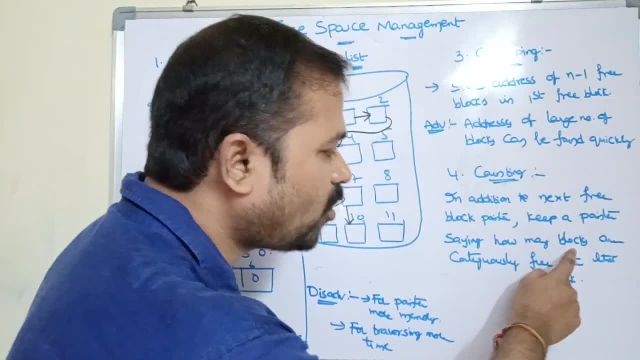 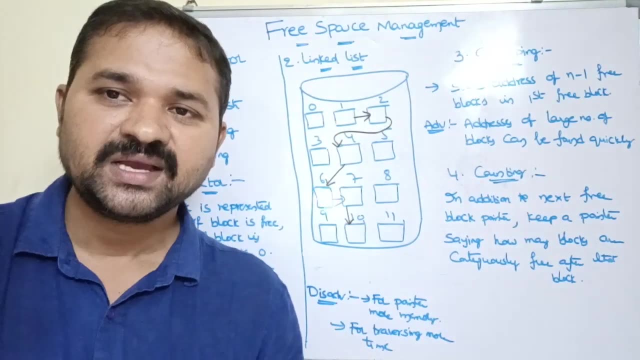 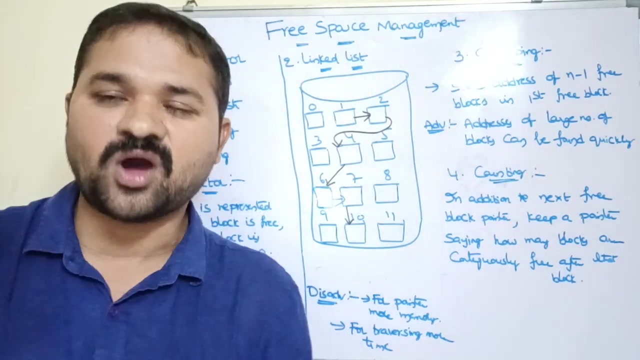 keep a pointer saying how many blocks are continuously free after that block. so it is also a slight modification to the linking list approach. in linked list approach, in each block we are maintain a pointer. that pointer contains address of it's next free block. in addition to that, it is better to